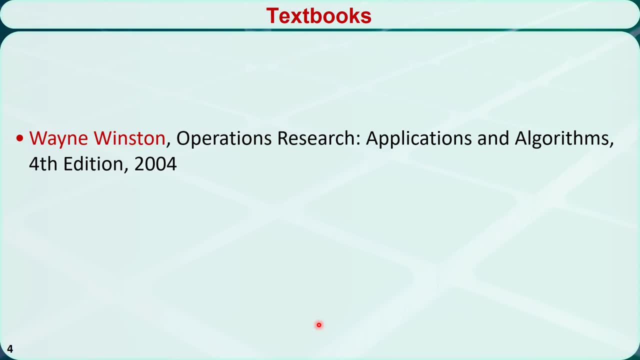 used in many universities in the United States. Two other great textbooks are Introduction to Operations Research by Healier and Lieberman and Operations Research- An Introduction by TaHa. It is highly recommended to have a textbook for reference when you are taking this course. Any one of these three textbooks. 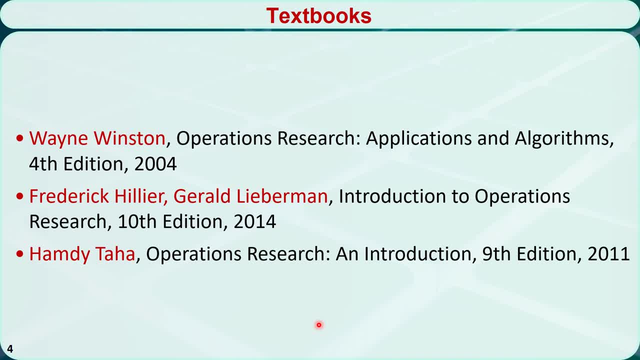 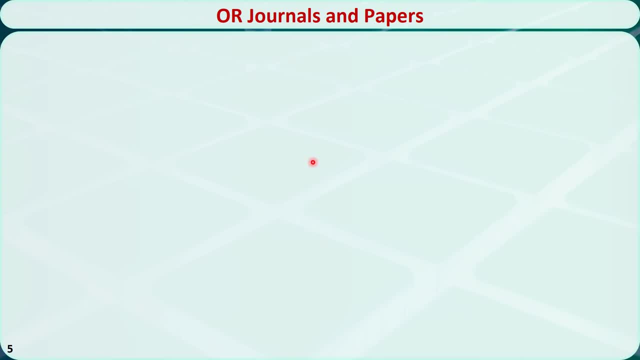 will do the job. If you are a graduate student or interested in the most recent theoretical development and application of operations research, you are encouraged to view this course and find out more about operations research, read and publish research articles in academic journals in this area. 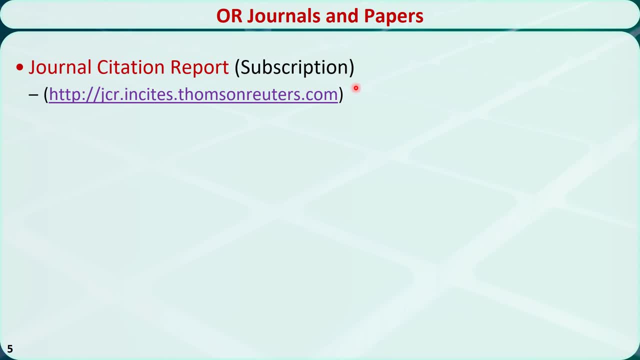 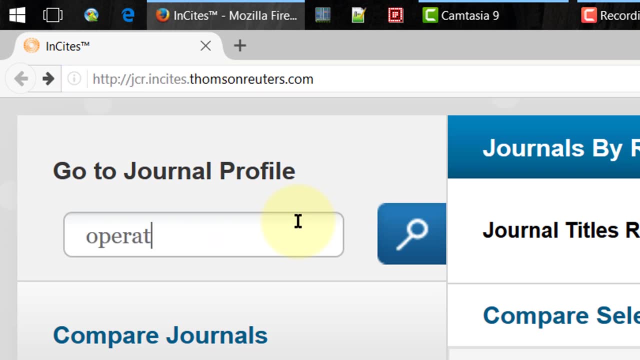 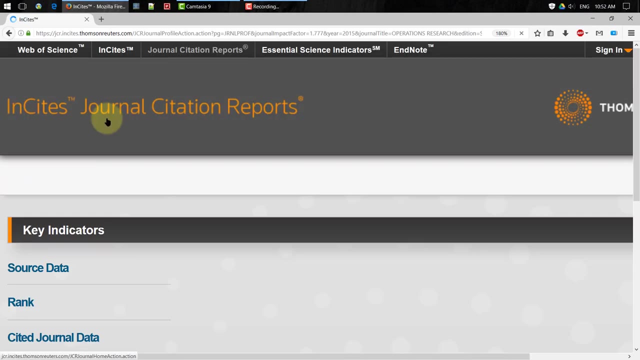 You can use a tool called Journal Citation Report to find relevant journals. For example, when you open this website, you can type in Operations Research, which is the journal's name, and click the first item. It will show you the detailed information about this journal. 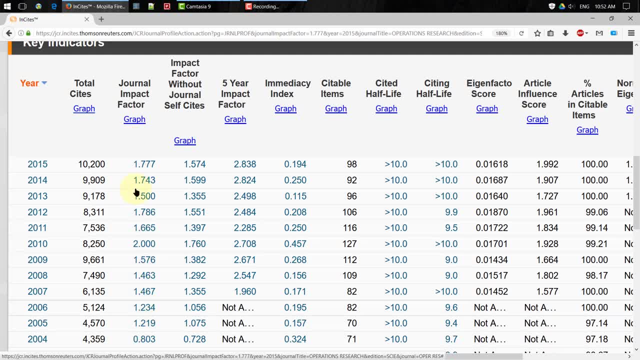 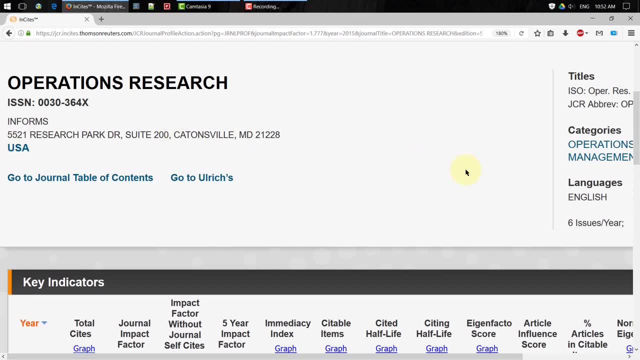 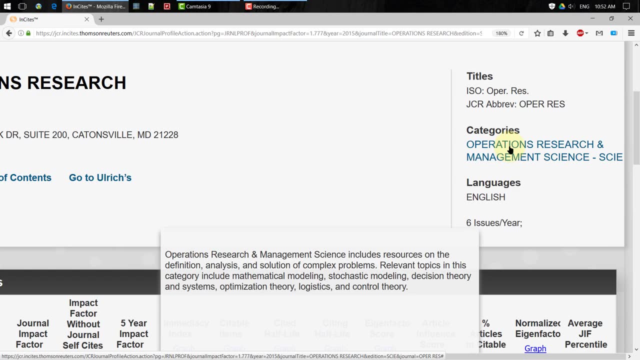 The most important one is probably the Impact Factor. The higher the impact factor, the more citations each paper gets in this journal on average. On the right column you can click this link under Categories. It will bring you to a list of journals related to Operations Research ranked by the impact. 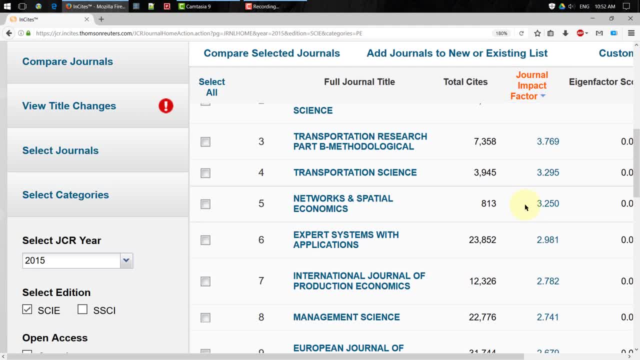 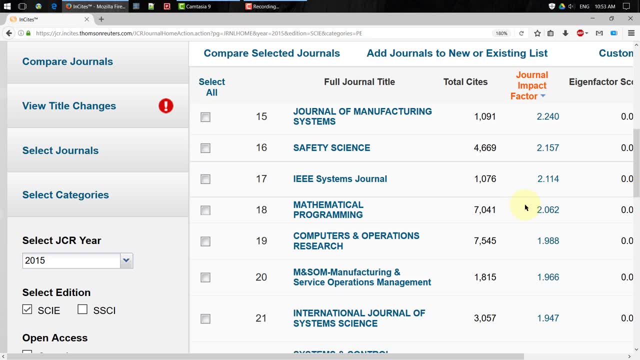 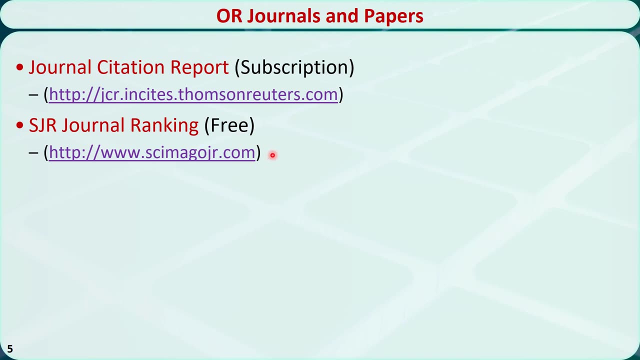 factors Journal Citation Report. requires you to need to write a list of the following References, titles and citations. requires that your university has subscribed their database and pay an annual fee so you can have access to the data. A free substitute is called SJR Journal Ranking. 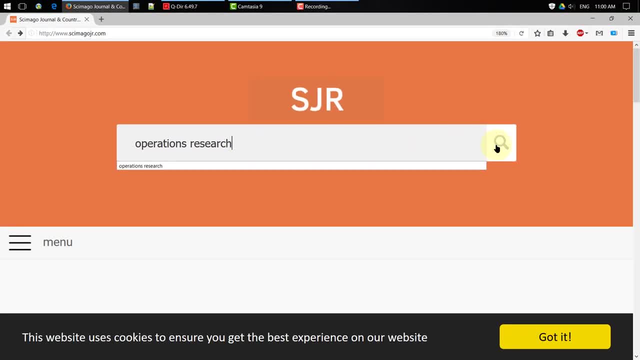 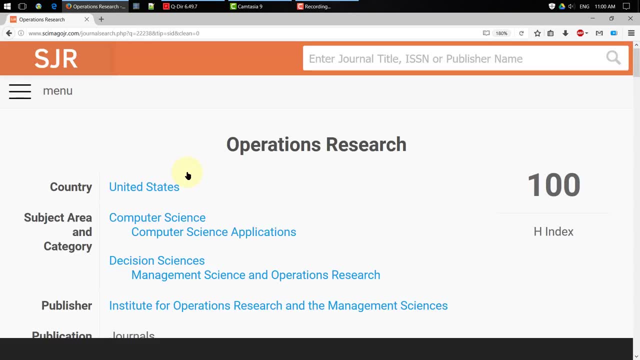 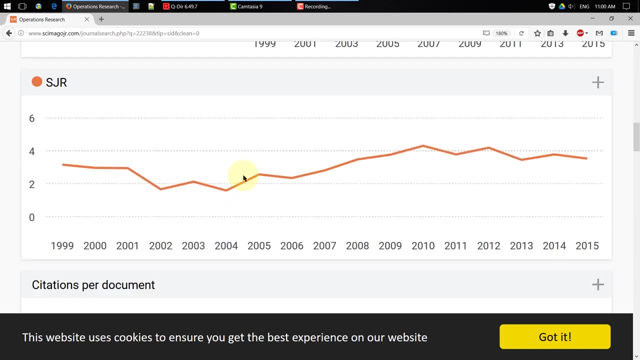 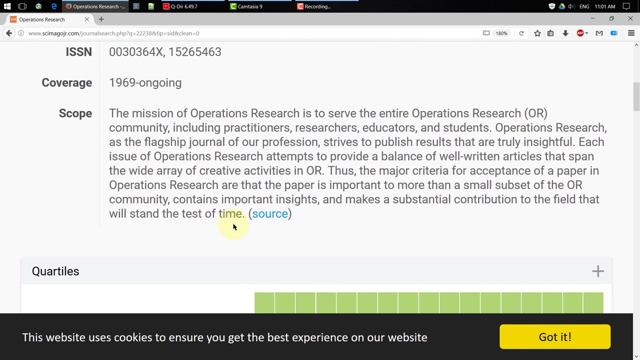 When you open this website, try to type in operations, research and click this search button and then select this journal. It will show you the detailed information about this journal. The most important one is probably the SJR index. The higher the SJR index, the more citations this journal gets. 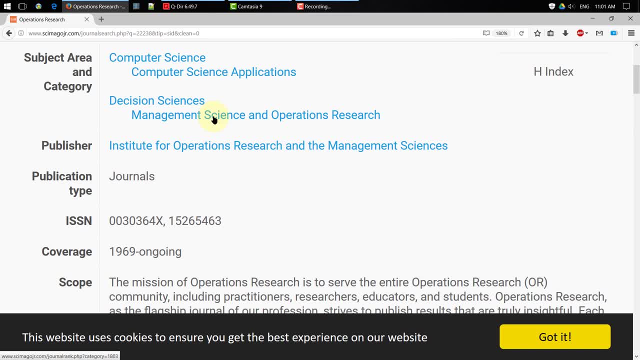 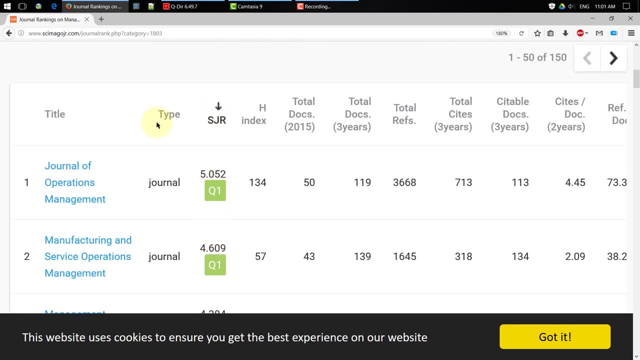 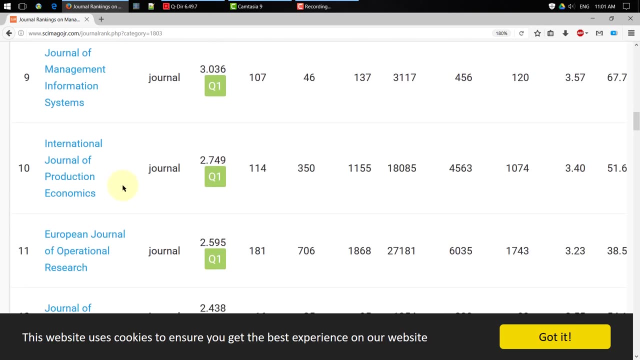 You can click this link: Management Science and Operations Research, enter subject, area and category. It will bring you to a list of journals related to operations research, ranked by their SJR index. This website uses different measures to rank the journals, So the rankings may be different from Journal Citation Report. 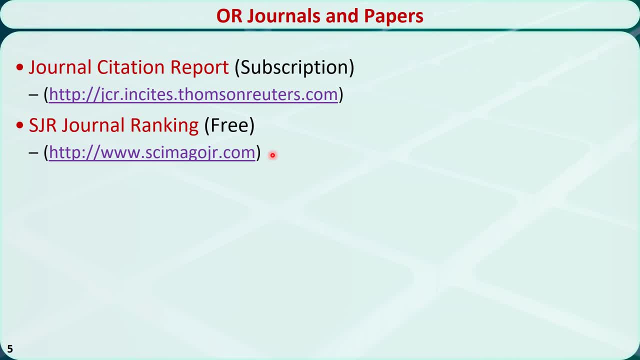 These tools are helpful to identify relevant OR journals. However, you should note that a journal will not be viewed the same by different industrial engineering departments at different universities. Even different professors in the same department may have different opinions about the ranking and reputation of the same journal. 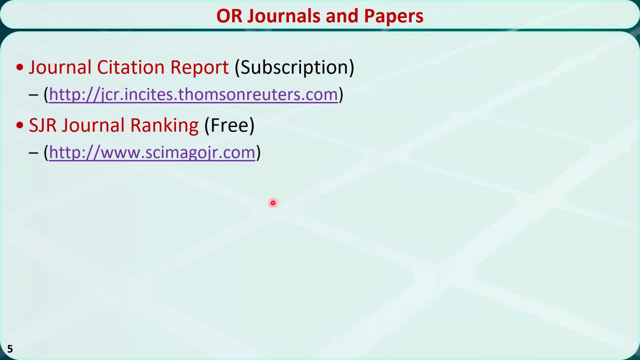 Students are encouraged to discuss this with their professors. 3. In order to download the full-text papers, you can use some academic databases, such as the Web of Science and the Science Direct. They both require that your university has bought the access to the databases. 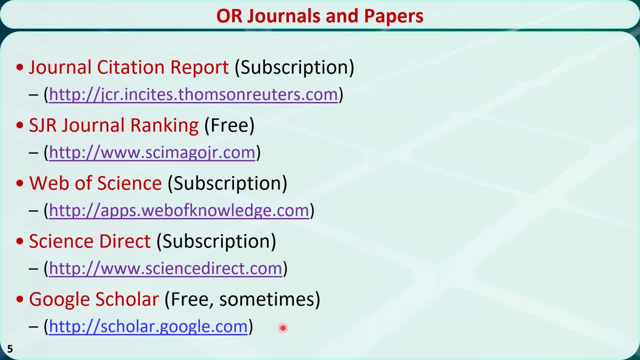 You can also use Google or Google Scholar to find a free copy of some papers. As a last resort, you can directly contact the authors of a paper you are really interested in but don't have access to for a free copy of the full-text paper. 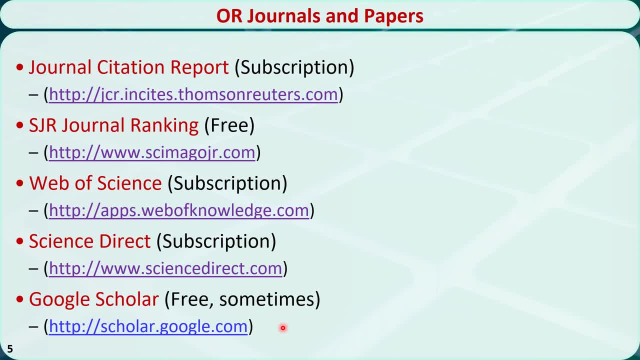 You can also use Google or Google Scholar to find a free copy of some papers. You can also use Google or Google Scholar to find a free copy of the full-text paper. Based on my experience, most people are willing to share their work. The links to these websites are put below this video. 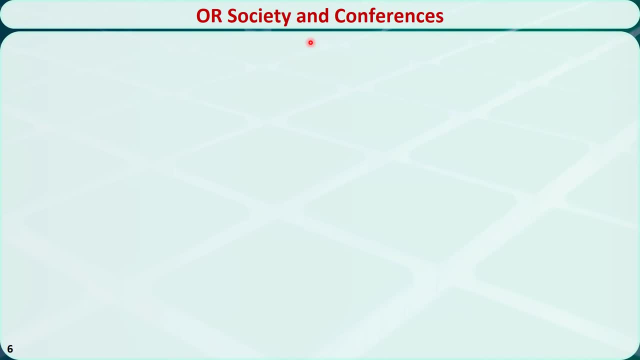 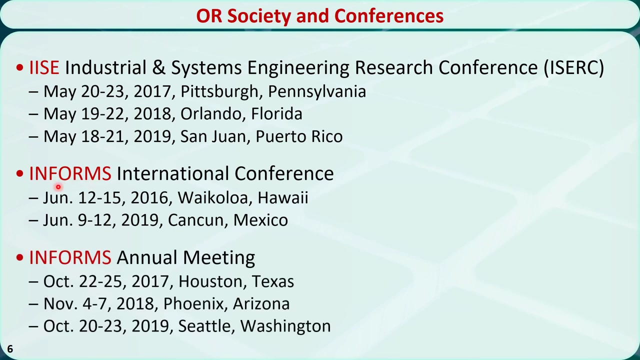 There are many operations, research societies and associations around the world, For example, the Institute of Industrial and Systems Engineers, or IISE, and the Institute for Operations Research and Management Sciences- INFORMS- Thank you. They organize international conferences annually So students, faculty from academia and researchers from industry will have the opportunity to 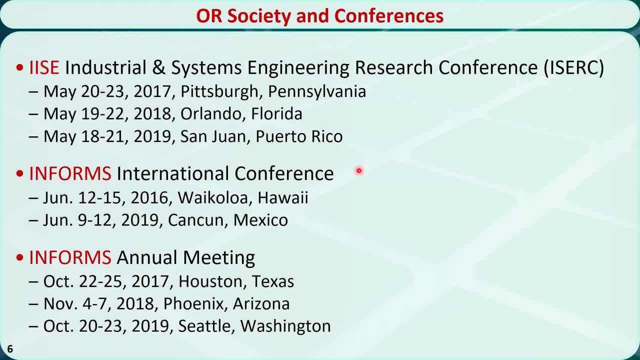 meet and discuss recent advances in this field. Many conferences are held in very nice places like Orlando, Florida, San Juan, Puerto Rico, Waikoloa, Hawaii and Cancun, Mexico. Many students are invited to the conferences. They are also invited to the conferences. 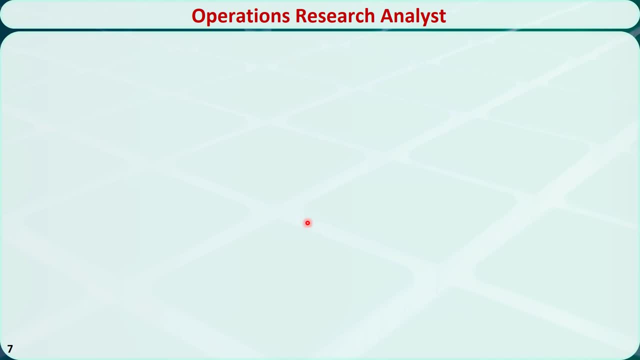 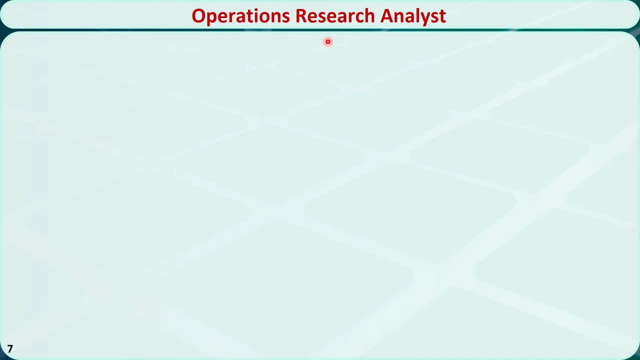 OR is one of those courses that are directly driven by industry needs. There is a specific job title for that. It is called Operations Research Analyst. You can search this job title at Indeedcom, which is one of the most popular job listing websites in the United States.